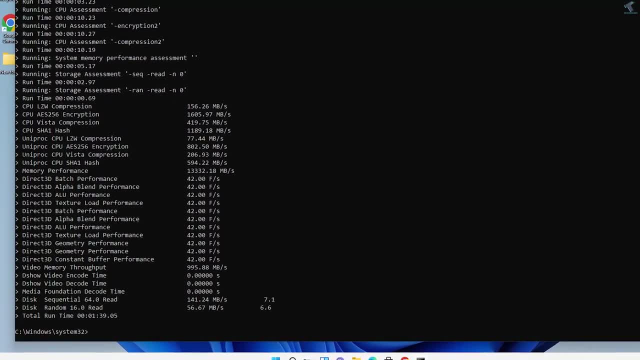 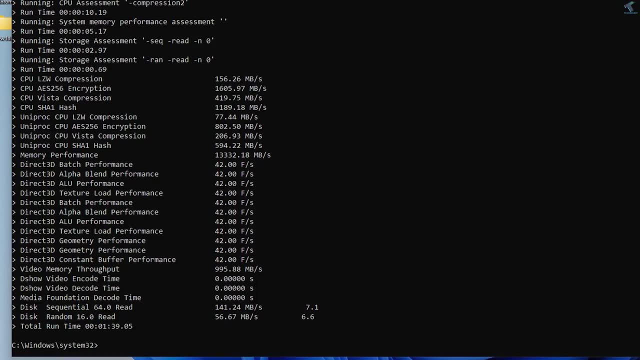 hi guys, welcome back to my channel technology, and today, in this video tutorial, i will show you guys how to run computer performance benchmark test on your windows 11 pc or laptops, so you just need to follow me. so at first you just need to go to your start or search menu. 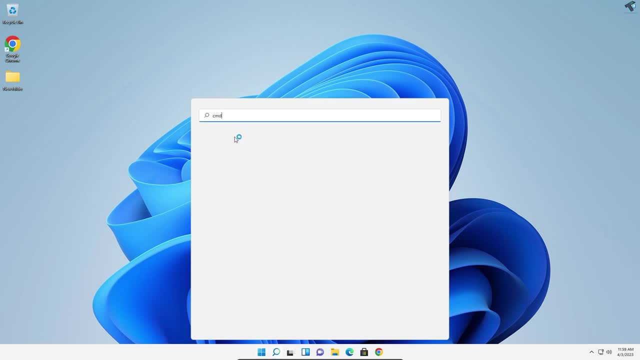 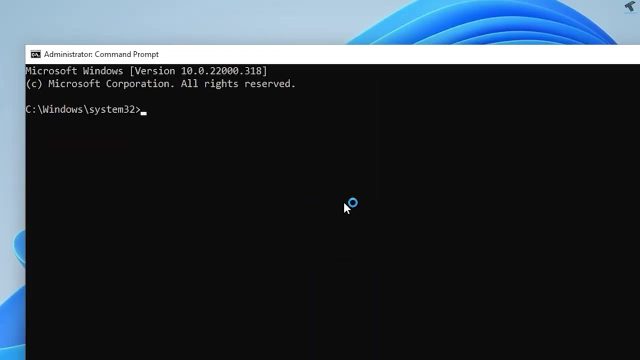 and type over here: cmd now. right click on command prompt. so just again right click on cmd, click on run as administrator. you have finished. now you click on éditorompter and get options. after that click on yes. now, after opening cmd prompt window, you just need to type one command over here. 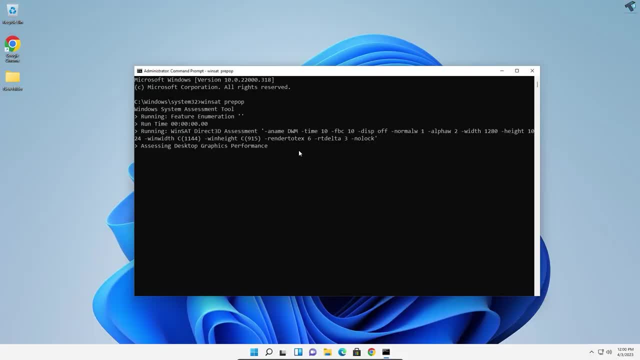 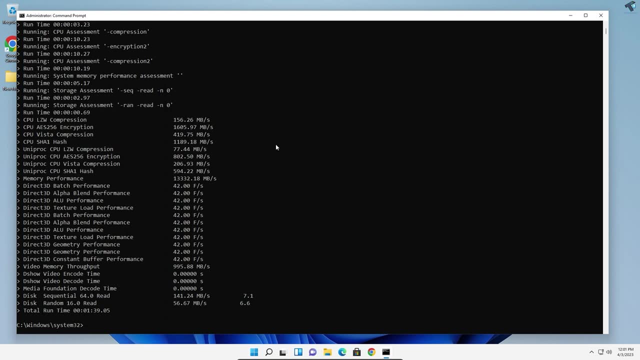 which is called win-set-prepop. After that, press enter from your keyboard. now it will take some time to analyze your hardware and it will give you the result. so i hope this quick tutorial is really helpful. yeah, any queries or questions in comments down below. I will see you guys in the next. video. till then, bye, bye, take care. 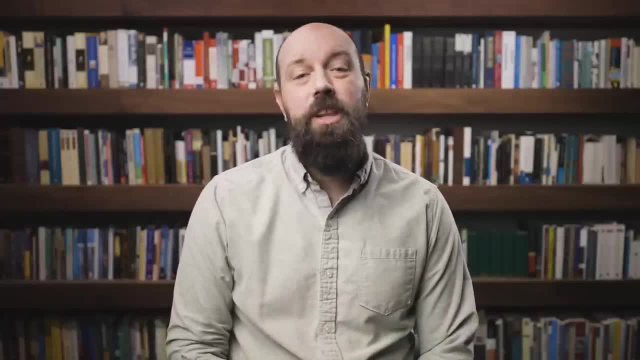 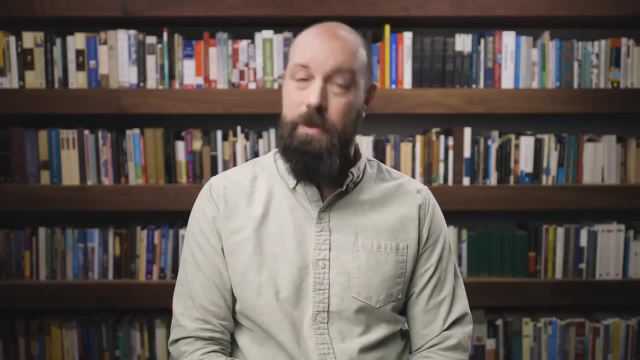 Hey there and welcome back to Heimler's History. Now we'll be going through Unit 4 of the AP Government Curriculum and in this video that means it's time to talk about the ideologies of the two major political parties of America: the Republicans and the Democrats. So if you're 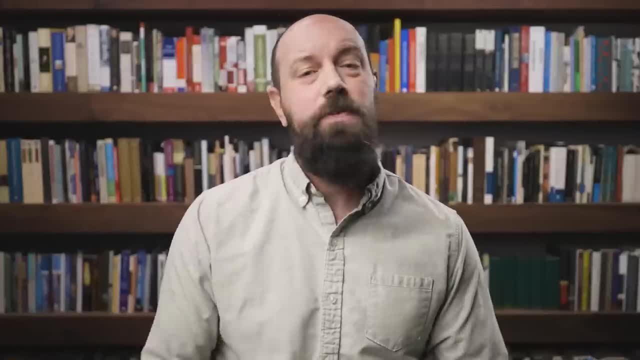 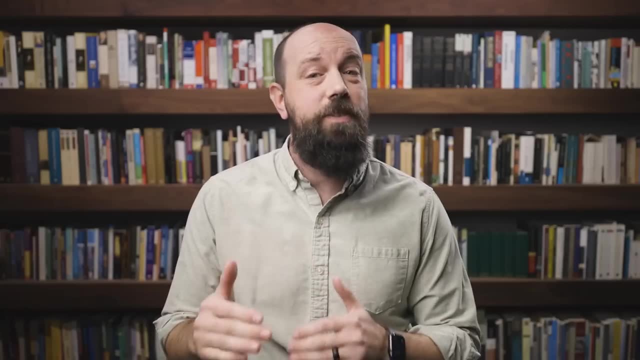 ready to get them brain cows milked party style. well then, let's get to it. So in this video, here's what we're trying to do: Explain how ideologies of the two major parties shape policy debates. Okay, so that means before we start talking about individual parties. 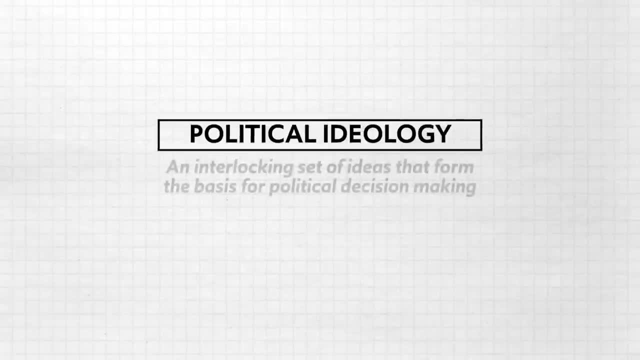 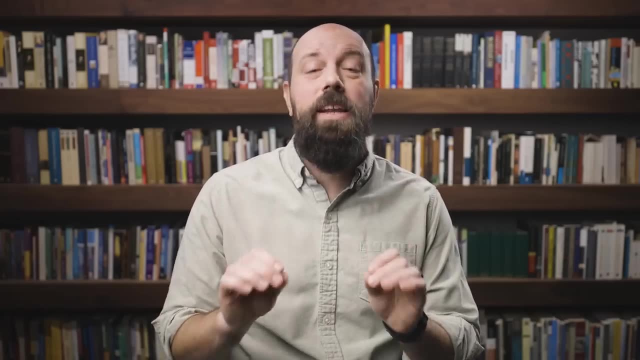 we need to understand political ideologies. A political ideology is an interlocking set of ideas that form the basis for political decision making, And, although what I'm about to say is a simplified version of reality, political ideologies basically fall along a spectrum between liberal and conservative ideologies. Now, conservative ideology emphasizes: 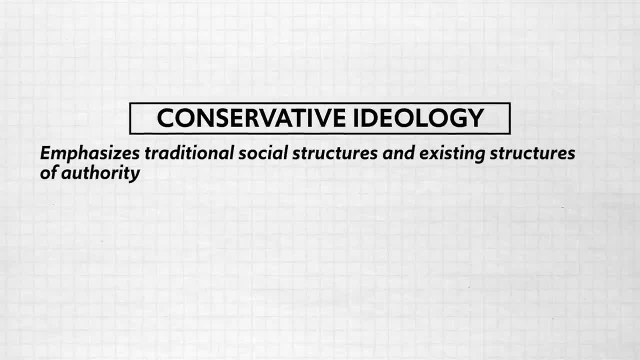 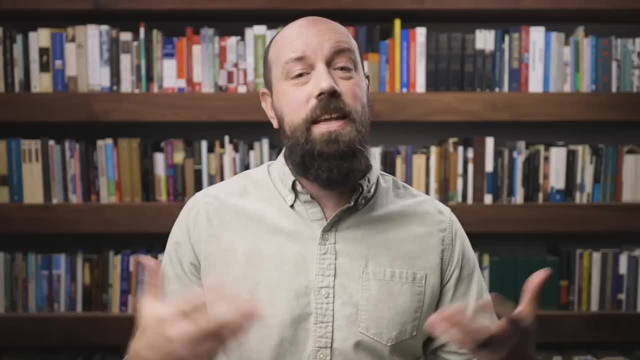 traditional social structures and existing structures of authority. Conservatives tend to emphasize limited government and public affairs, strong stances on crime and punishment, and champion states' rights over federal power. Or to say it another way, conservatives look at what exists and say: if it ain't broke, don't fix it. Liberal ideology, on the other hand,